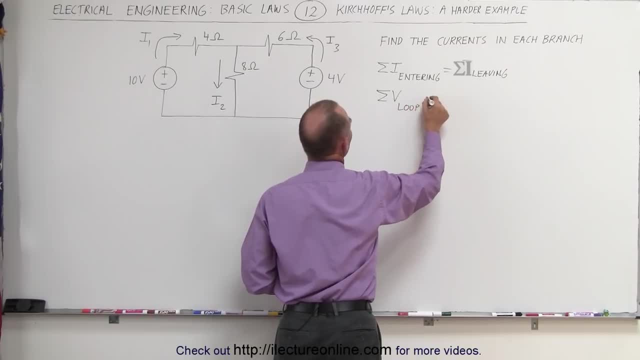 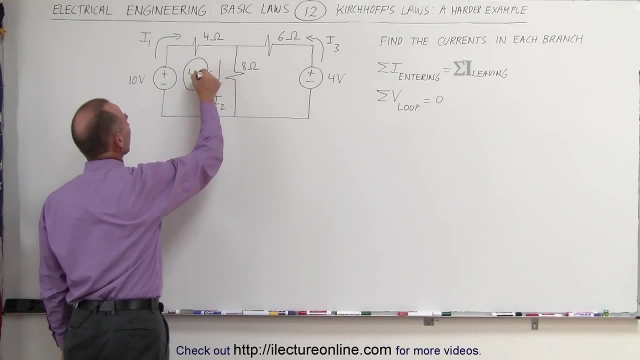 sum of all the voltages around in a loop should add up to zero. We're going to use two loops. Here's loop number one. It's always a good idea to indicate the direction that you're taking when you're going around the loop. And here that's loop number two. And again, 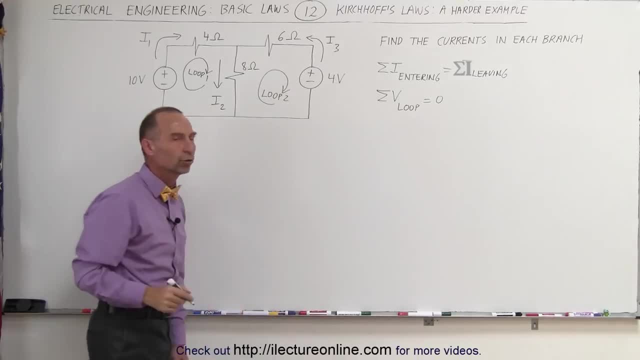 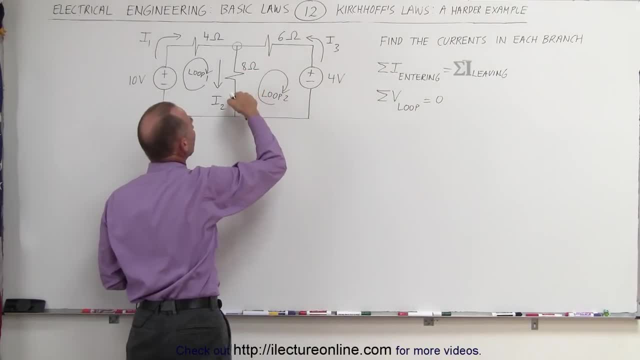 going to add up to zero. So I'm going to add up to zero. So I'm going to add up to zero. And here's loop number two: I1 plus I3 add up to I2.. These are the two currents entering. 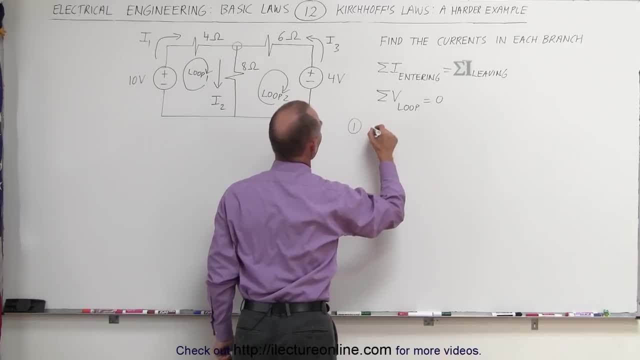 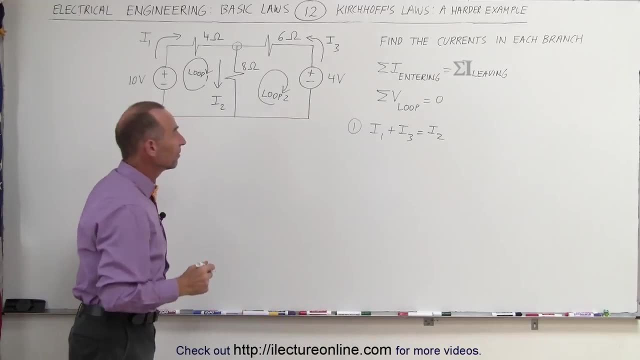 the node and one current leaving the node. So equation number one tells us that I1 plus I3 equals I2.. The second equation can be found by going around loop number one. I can start at this node right here. go around loop number one, get to the same node and add up all. 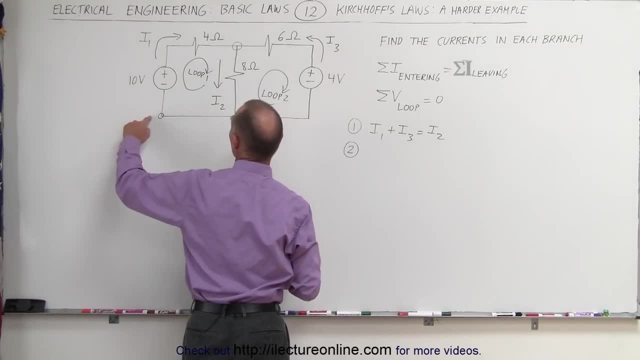 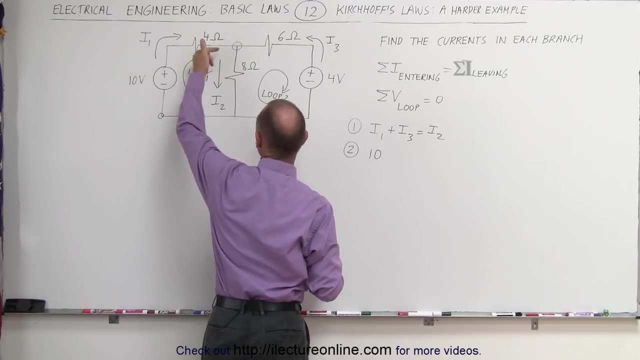 the voltages. So equation number two is obtained by going from here to here- And here I'm coming from here- across the battery, from negative to positive, that's a positive 10 volts. Going across the resistor in the same direction as the current means we have a voltage. 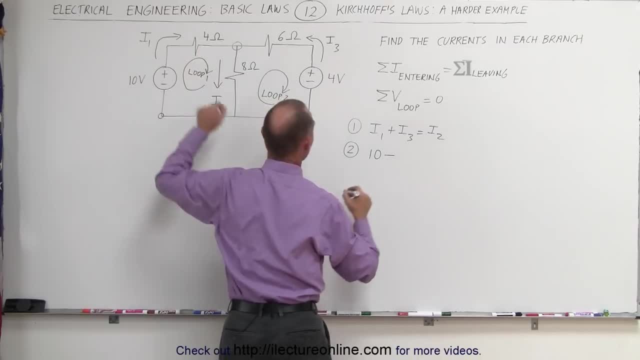 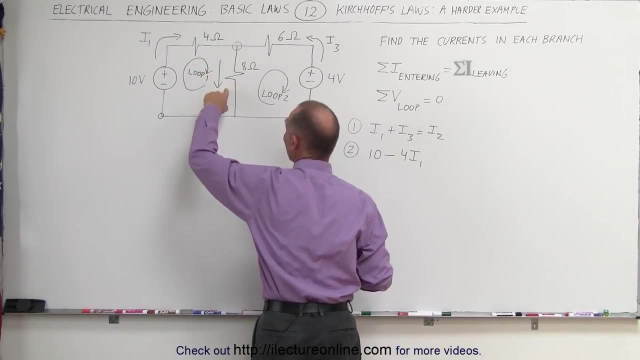 drop. so we get minus four times I1.. Coming down through this branch here in the same direction as the current—that's another voltage drop—minus eight times I2.. Then I get back to the same point where I started. so therefore this should add up to zero, That's. 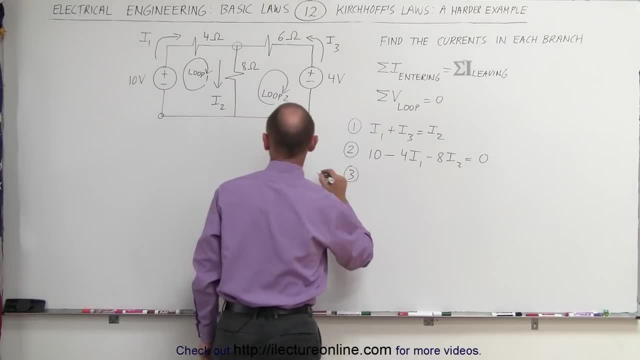 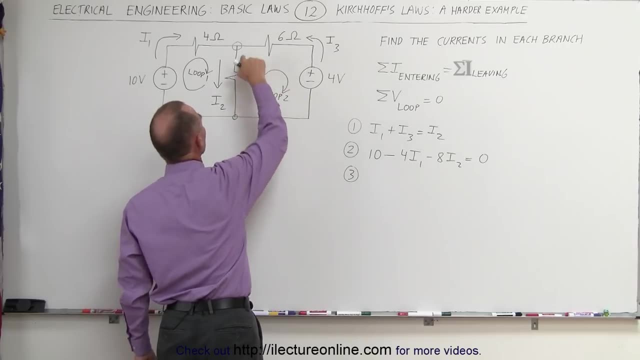 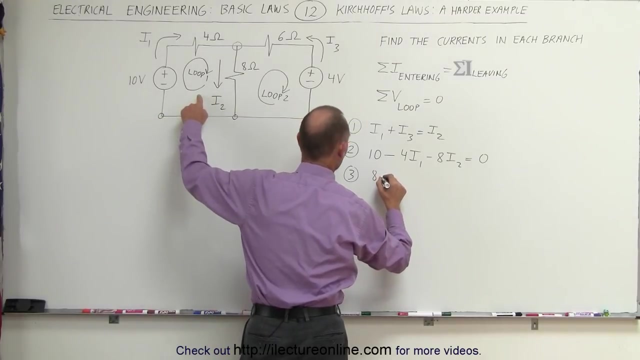 equation number two. equation number three can be found by starting at any node in the loop. let's start with this node going from here in a clockwise direction across this resistor. against the current, that means that's a voltage rise that's plus eight times the current i2. then in this direction, that's. 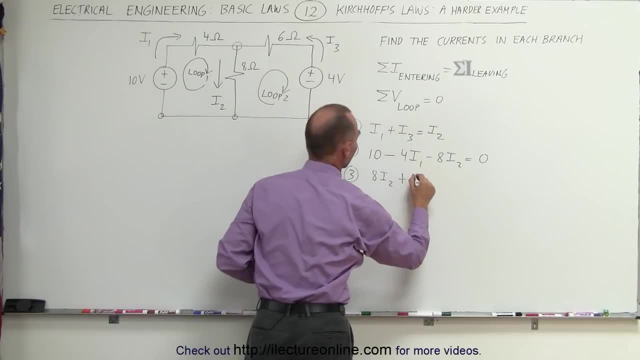 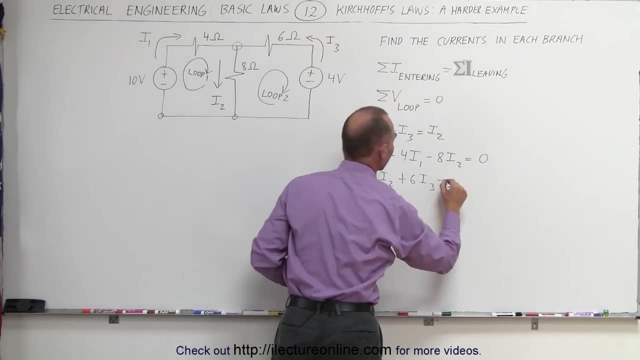 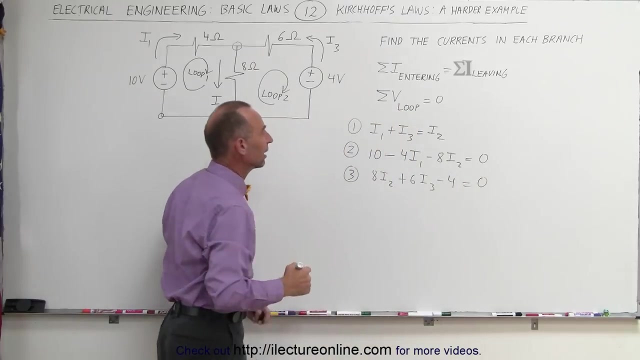 against the current, that's a voltage rise plus six times i3, and then from here to there, that's from the positive end, the negative end of the battery, that's a minus four volt drop. we don't have to write the units to say four, and since we can then get back to the same point, that adds up. 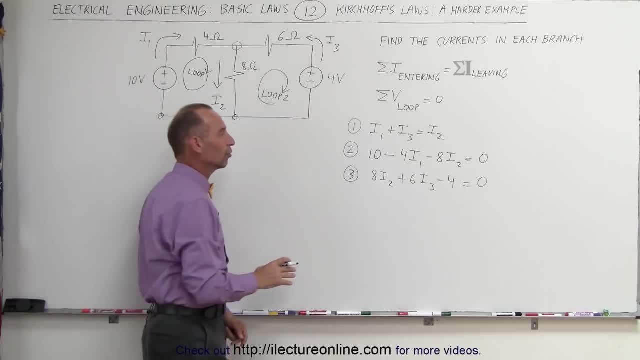 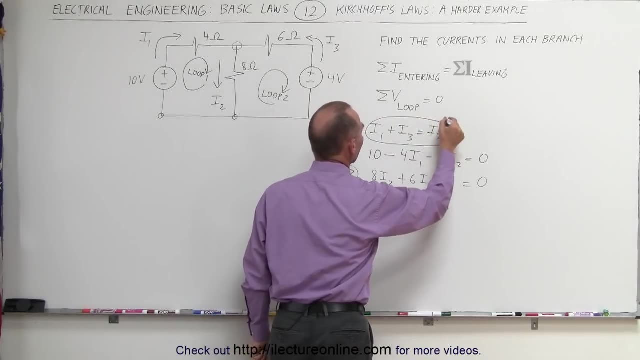 to zero. there's the three equations and we can use those to find the three unknowns: i1, i2 and i3. i like to use this equation first because it usually already has one of the currents in terms of the other two. we can take that to substitute that into this equation right here and into this. 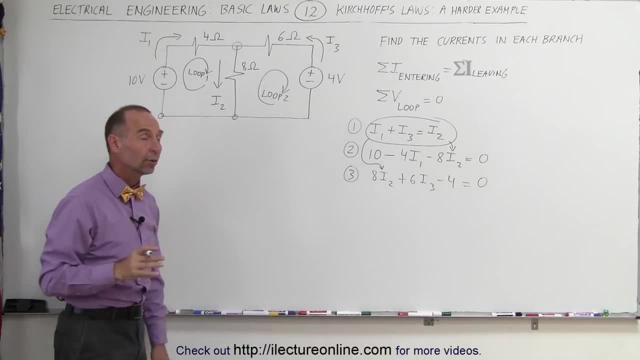 equation right there. so the the two equations, two and three, will now change to the following: two is now going to be equal to ten minus four times i1 minus eight times, and instead of writing i2, we can write i1 plus i3, i1 plus i3. the third equation, same thing. instead of writing i2, i can write i1 plus i3. this gives me: 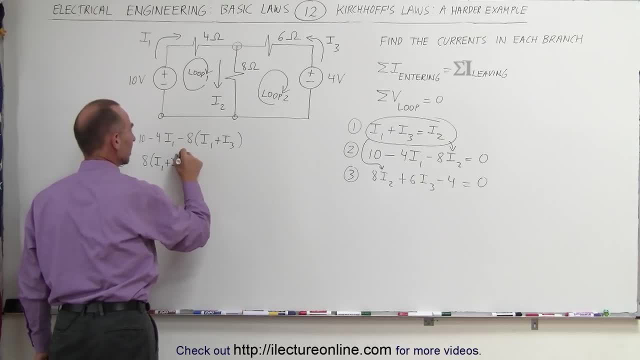 eight: i1 plus i3 plus six, i3 is equal. oh, not equal. yet minus four is equal to zero. simplifying the two equations, writing all the i's on the left side and all the constants on the right side, equation number two. so we keep these two going. equation number two now becomes: 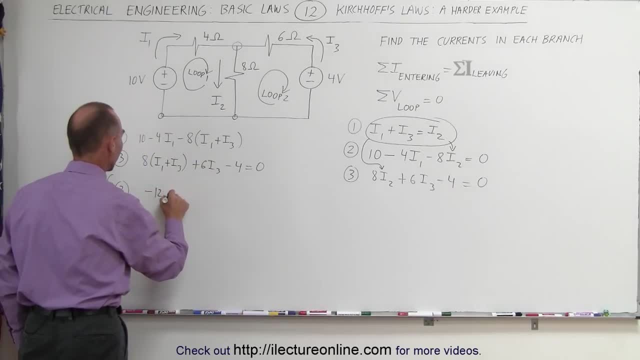 minus four. i1 minus eight. i1 is minus twelve. i1 minus eight times i3 is minus eight. i3 equals, when we bring the ten to the other side, becomes a minus ten. the third equation we have eight times i1, eight times i3 minus six, that's. 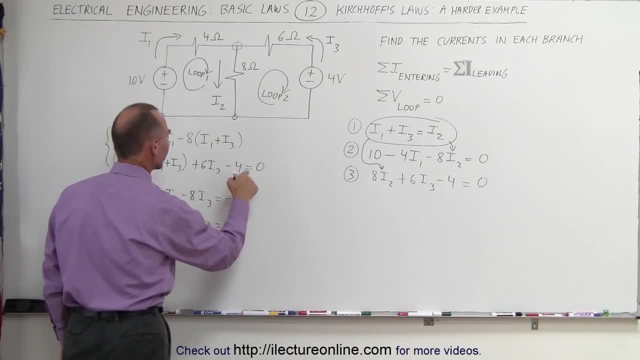 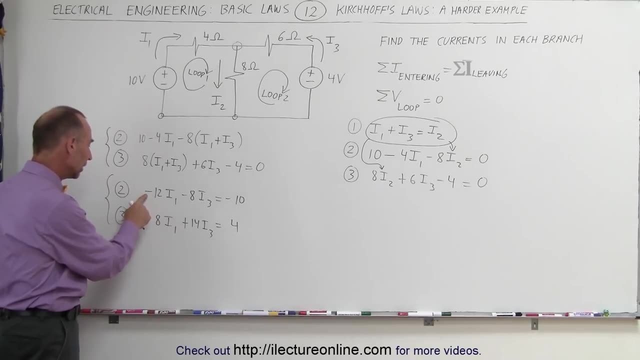 plus fourteen, i3. that equals. when we bring the minus four to the other side, it becomes a positive four. now notice that if i multiplied the second equation by two and i put the third of the two equation by three, then minus twelve becomes minus twenty four, then the eight becomes plus twenty four. when i then add the two equations together, 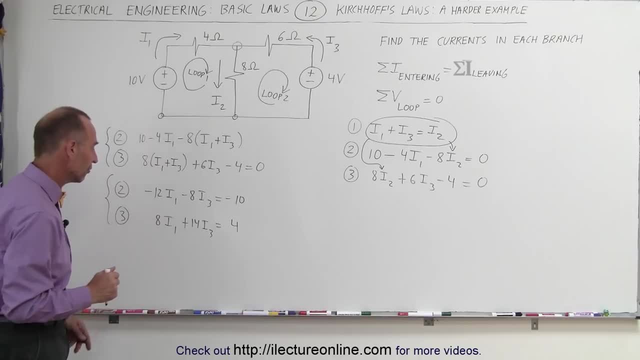 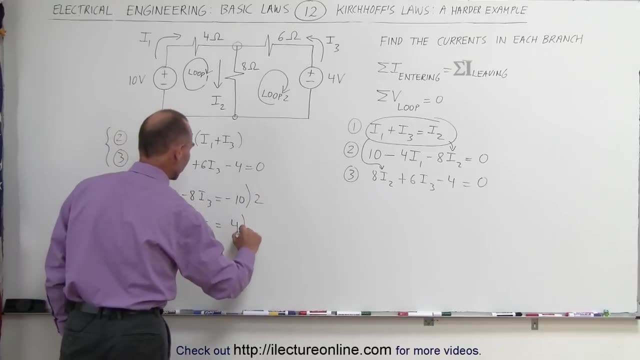 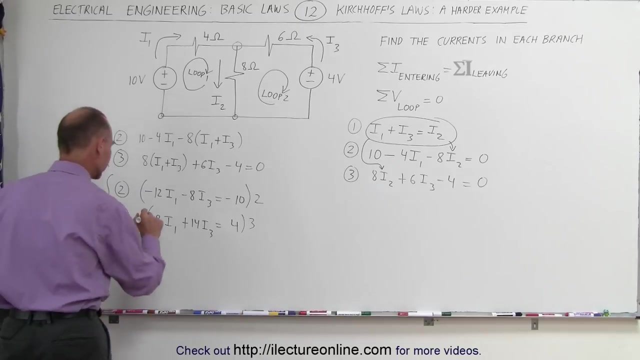 i1 equals two times 0. D ones drop out, and only I'm left with a single unknown which I can solve for. So the two equations now become as follows: I'm multiplying this equation by 2,. I'm multiplying this equation by 3 and I get. this is equation number 2, equation number 3, minus 24 I1, minus 16 I3. 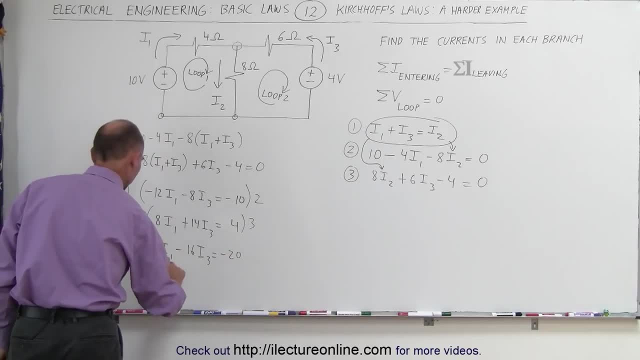 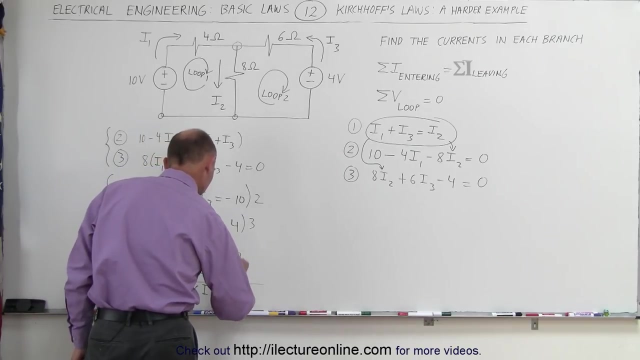 equals minus 20, and this equation plus 24, I1 plus, that would be 42. I3 equals plus 12.. When I add the two equations together, notice the I1's drop out: 42 minus 16, that would be 26 I3,. let's see: 26 plus 16, that's 42, and this becomes 20 minus 20 plus 12 minus. 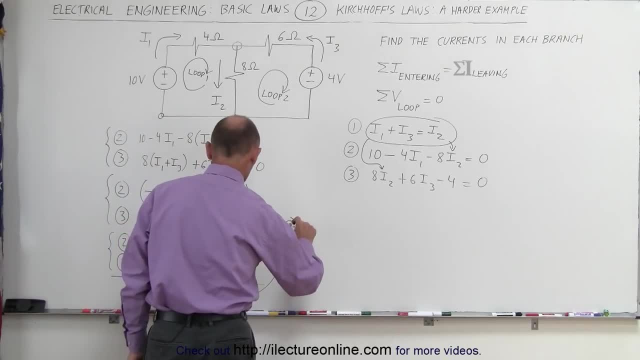 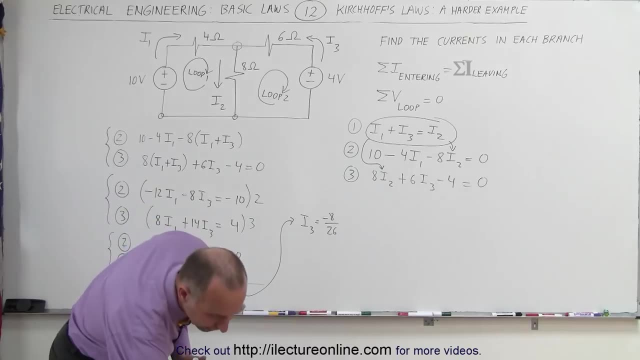 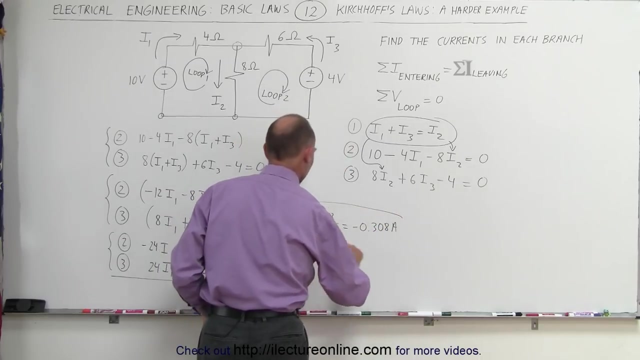 8. Which means that I3 is equal to minus 8 divided by 26,. and let me get a calculator for that: 8 divided by 26 equals 0.308, minus 0.308 amps. Notice that we end up with a negative. 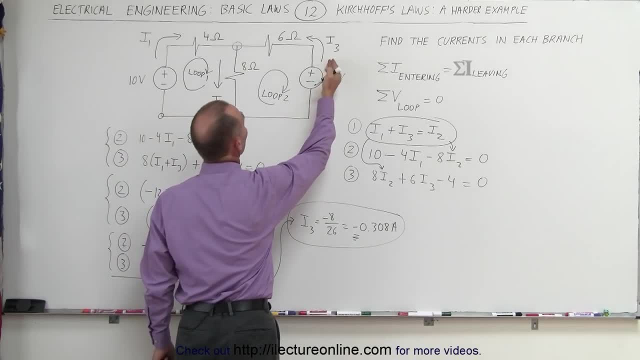 negative current, which means my initial assumption that the current was in a counterclockwise direction In this loop. it's actually in a clockwise direction, So the negative indicates that the actual current is in the opposite direction. But that's okay, we can leave it like that. 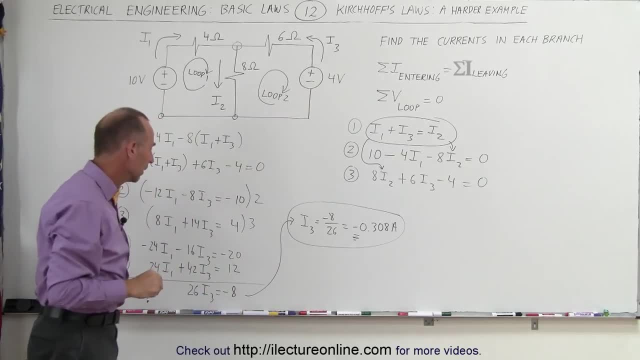 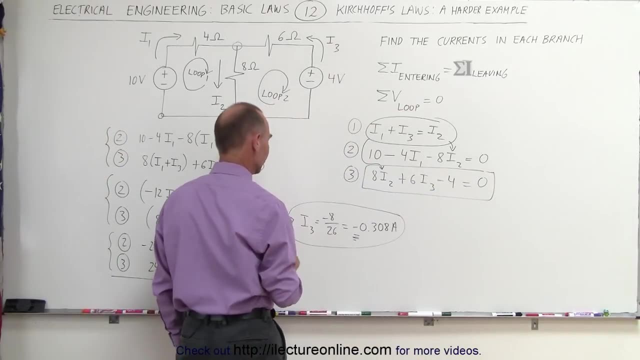 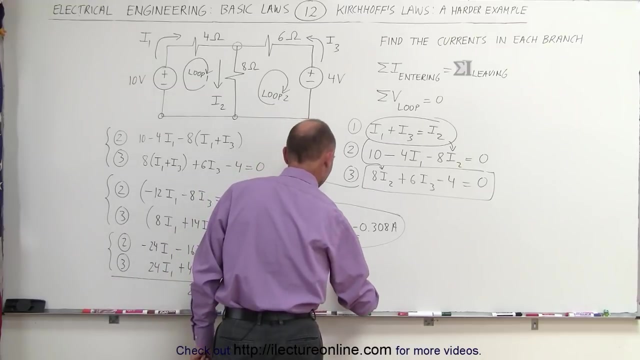 that we can then realize the current is simply in this direction. Now we need to solve for I2.. Let's use this equation right here to solve for I2.. 8 times I2, so I'm taking this equation over here: 8 times I2 plus 6 times I3, which is a. 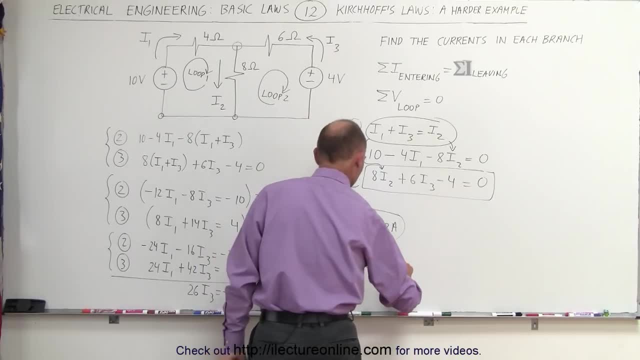 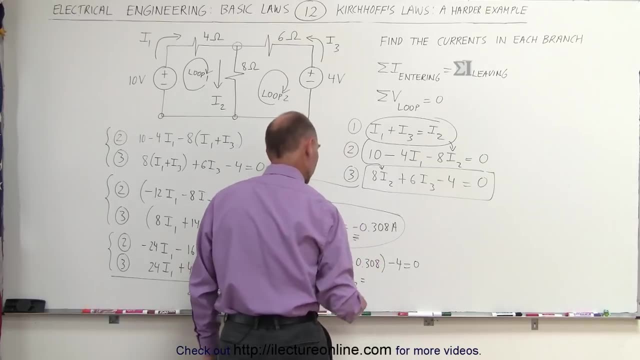 negative: 0.3. 0.3. 0.3. 0.3. 0.3. 0.3. 0.3.. minus 4 equals 0,, which means that 8 I2 is equal to positive 4 plus 6 times 0.308, and. 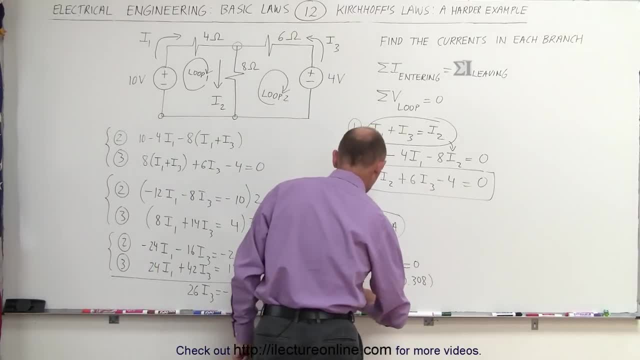 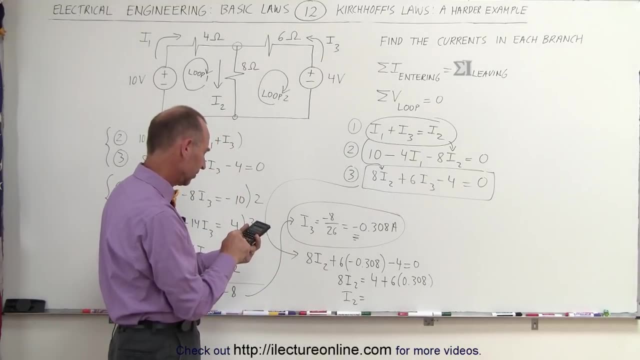 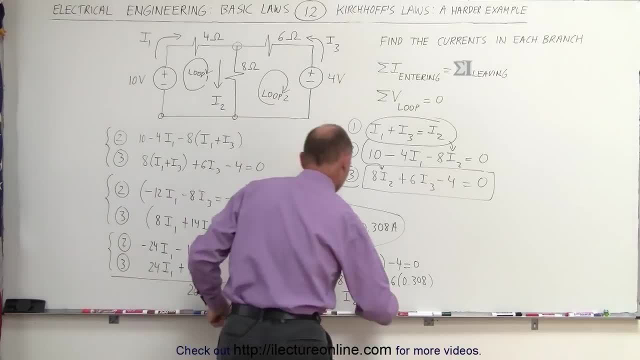 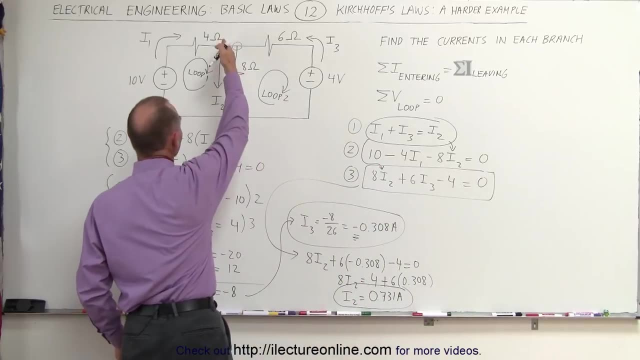 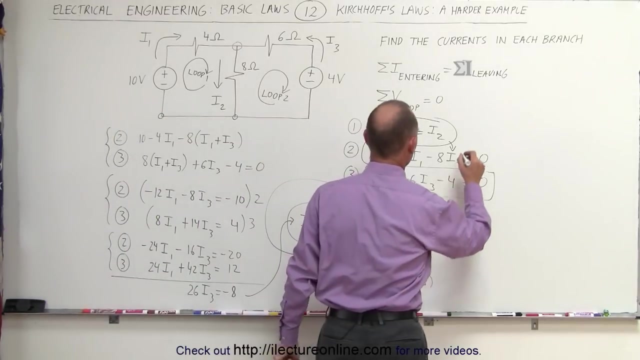 Okay, get 0.731, 0.731 amps, which is the current in I2.. So I2, I do have the correct direction because I got a positive answer. Finally, we can solve for I1 using this equation: I.